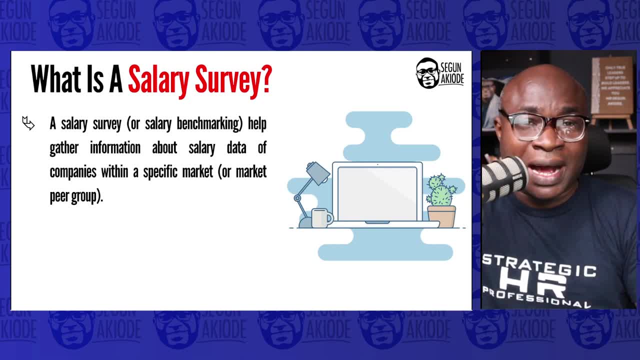 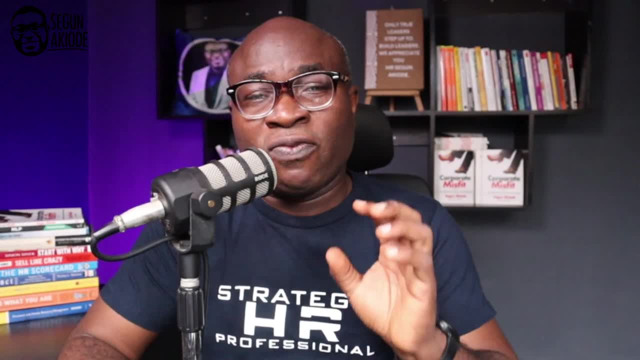 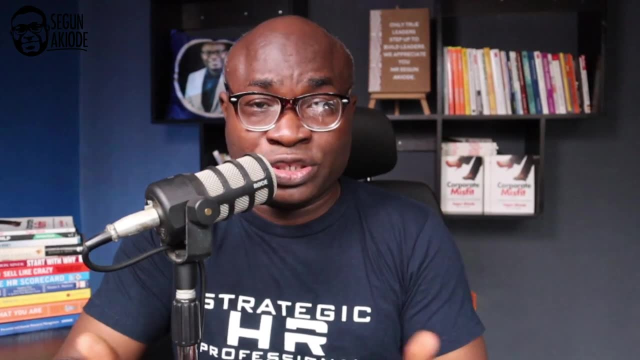 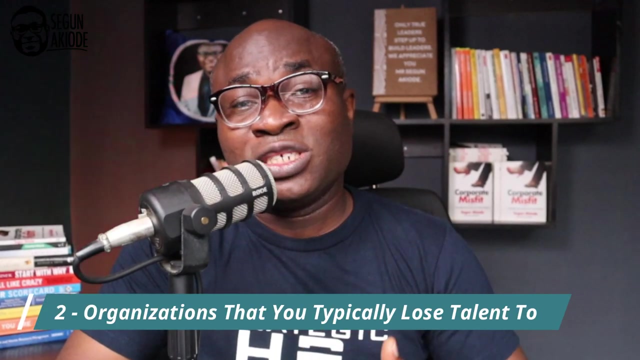 about companies within a specific market. That specific market is usually what we term your market peer group. The market peer group for any particular organization typically composes three different sets of category of organizations. Number one are organizations that you typically recruit staff from, Two organizations you typically lose staff to. And the third category is organizations that are in a similar industry doing something similar to yours, or organizations of similar size in another related industry. This will form your market peer group. Now, the reason why there is a need for a market peer group is that an organization cannot compete. 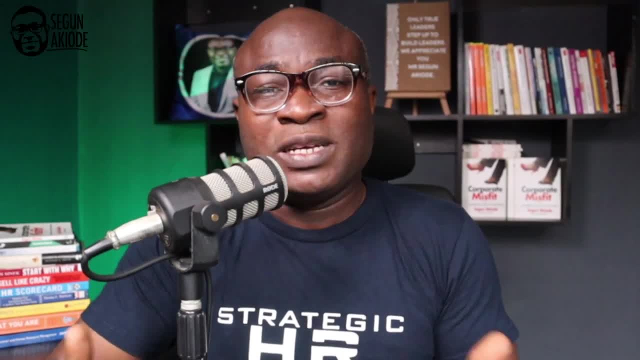 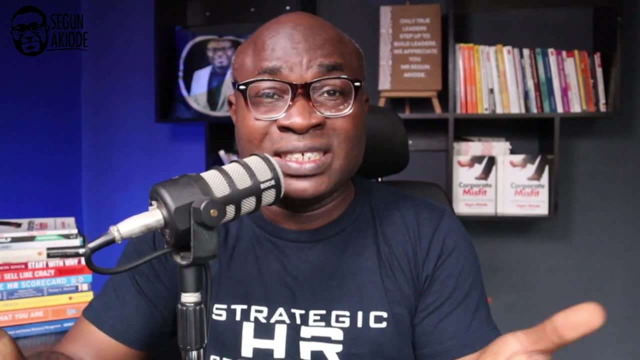 An organization cannot compete itself to the entire market. So typically your one organization, you're operating within a market that has 20 companies in that industry. If you compare yourself to the entire 20, then you're not being strategic. That's why there's always a need for a 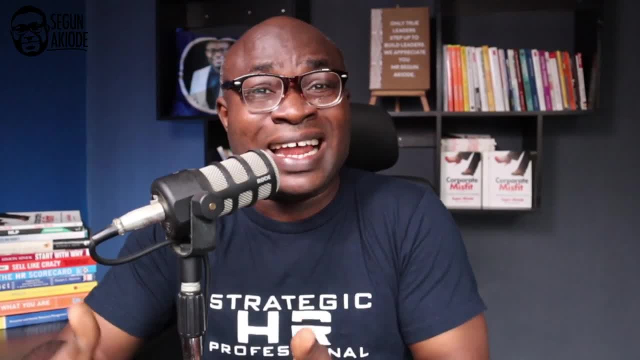 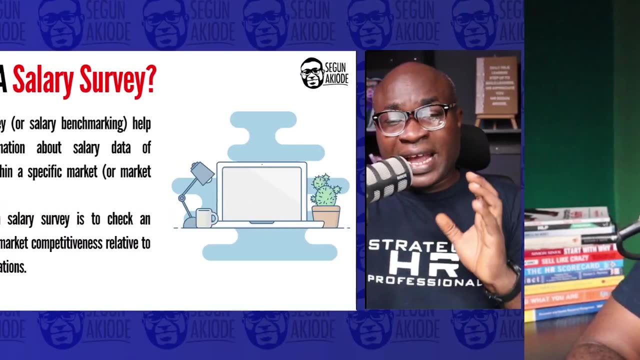 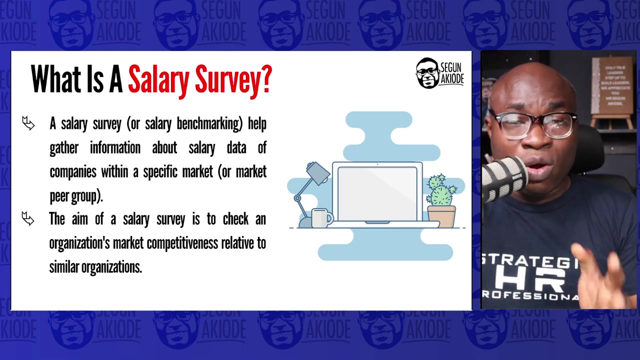 specific market peer group. That peer group must be selected by that organization. The essence of the selection is to be sure that you're comparing apples to apples. The aim of salary survey is to compare organizations' market competitiveness relative to similar organizations, which is the 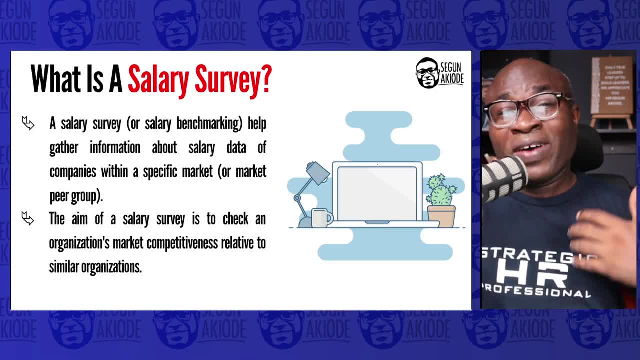 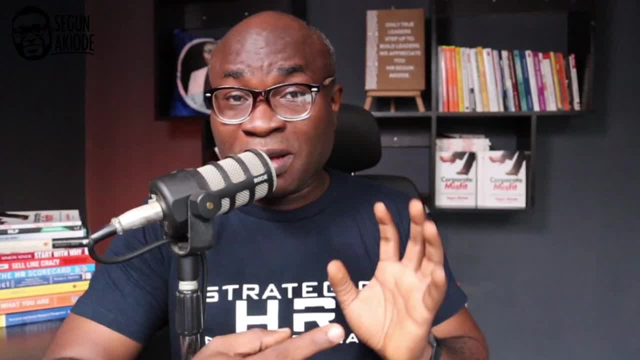 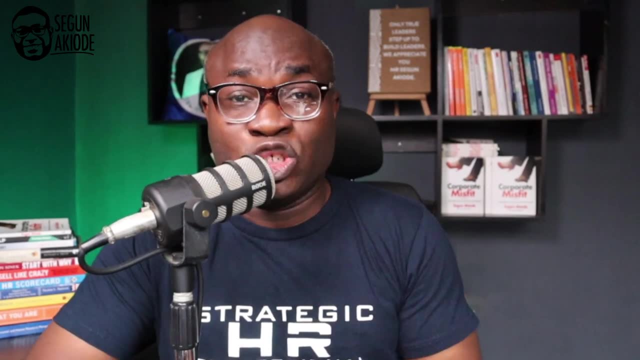 peer group that have been defined. This is where the concept of external competitiveness comes into play. After gathering the salary data from the market peer group, there are a lot of processes that this involves. One is doing what we call a job matching. Job matching is deciding what are 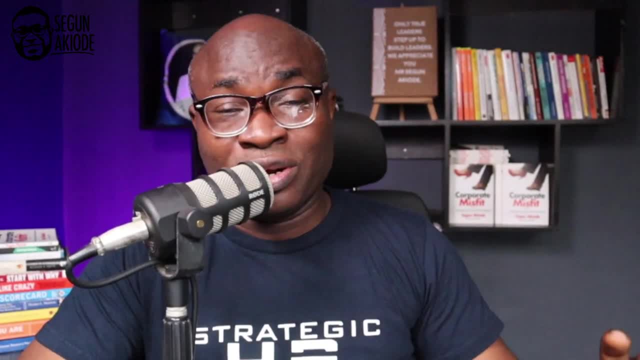 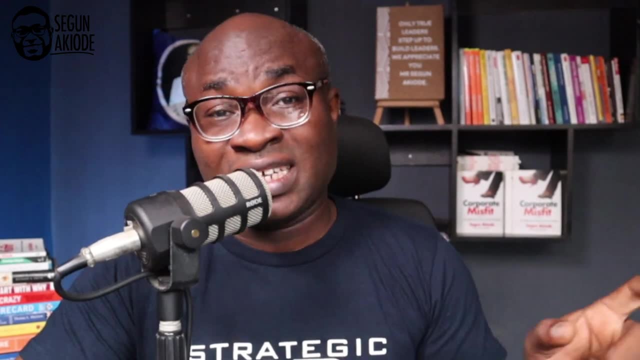 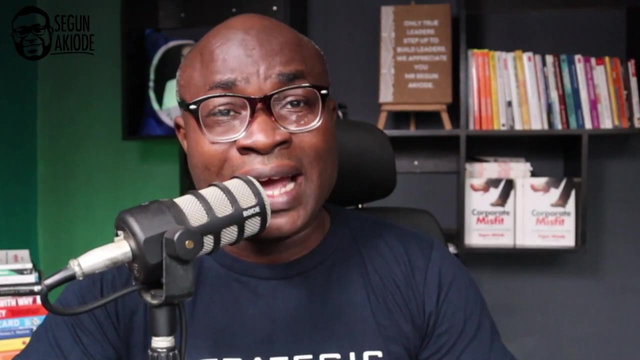 the benchmark jobs that we're going to compare across the organizations that we have defined as our market peer group, Because those are the jobs that would serve as a common element of what we call the survey levels that we want to check for. Then you will go ahead to gather the data. 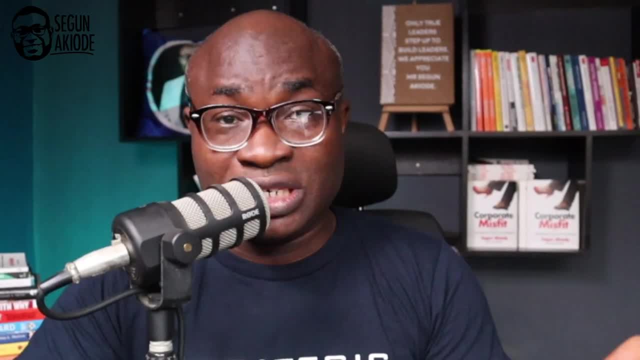 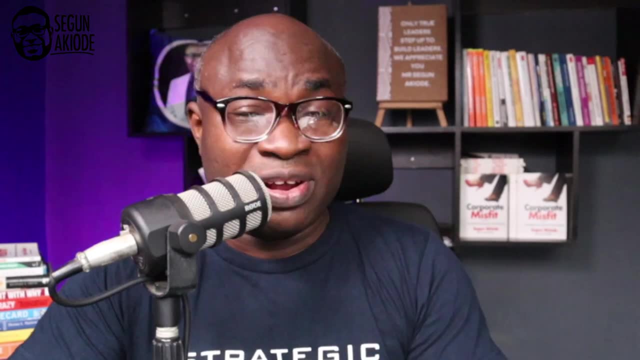 Gathering the data means you're defining: what kind of data do you need? Do you need only fixed pay from that organization, Or you need, how they undo, variable pay, or what we call your short-term incentive, your long-term incentive? how do they? 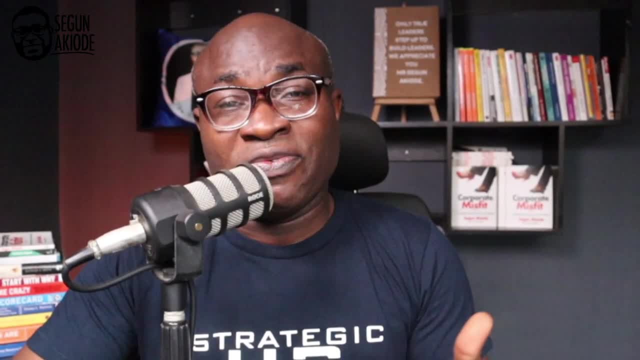 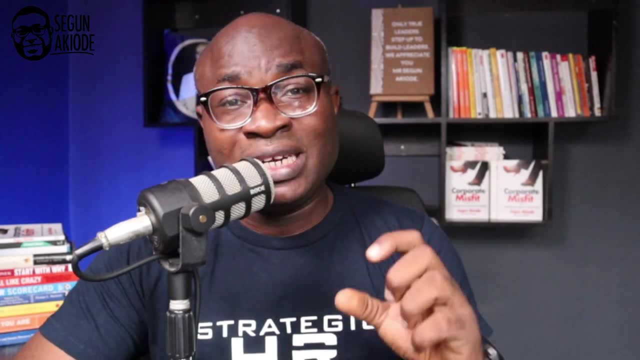 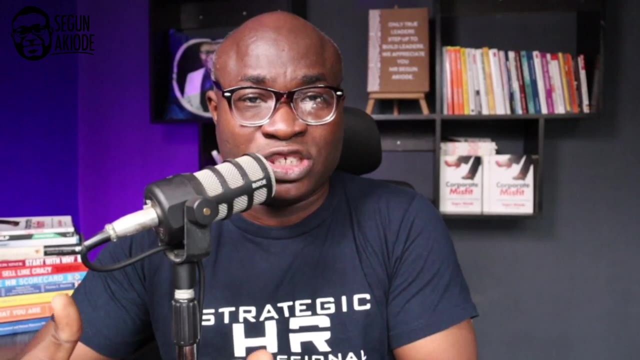 undo retirement benefit and all those conversations around benefit in kind. Now, after all of that has been collected, you now need to interpret. Interpreting means you're deciding what we call our external competitiveness, what's going to be our compensation philosophy. 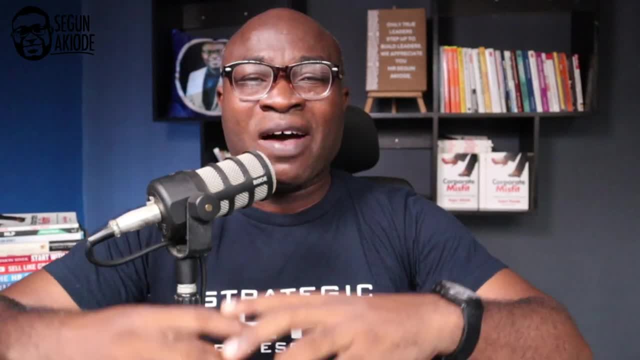 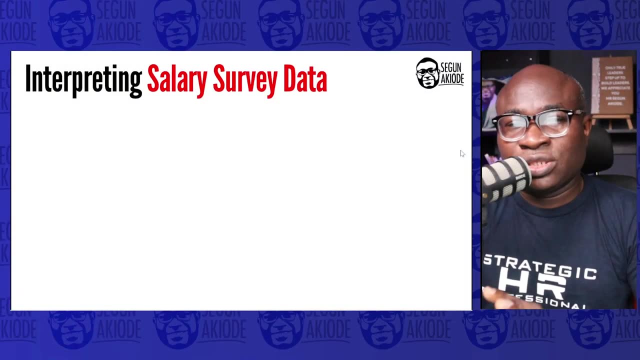 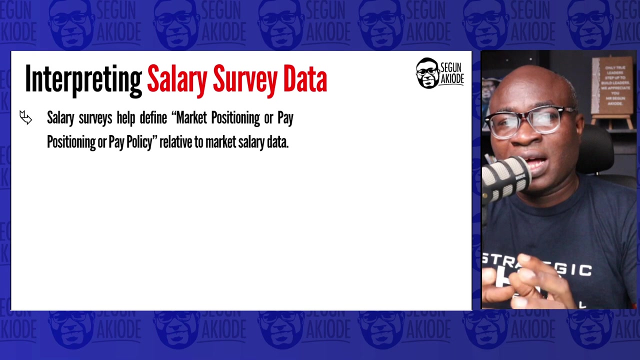 or what we call your pay policy. So now, after getting all this data from our similar markets, what are we going to do with this data? Now let's get into interpreting salary survey data. Now for you to be able to interpret the salary survey data, the salary survey data is: 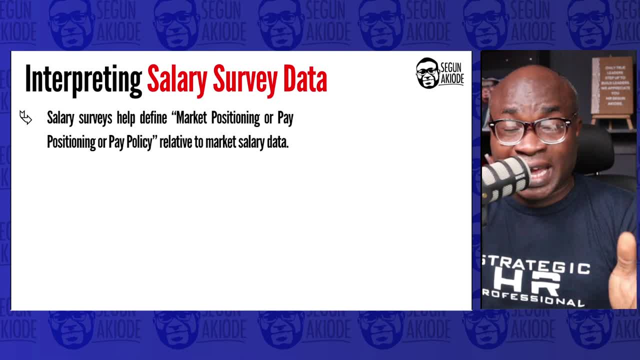 critical in helping organizations to define their market positioning, or what we often call their pay positioning, of the pay policy line. Now, the pay policy is usually relative to the market salary data, and there are three major positions that an organization should be able to do. 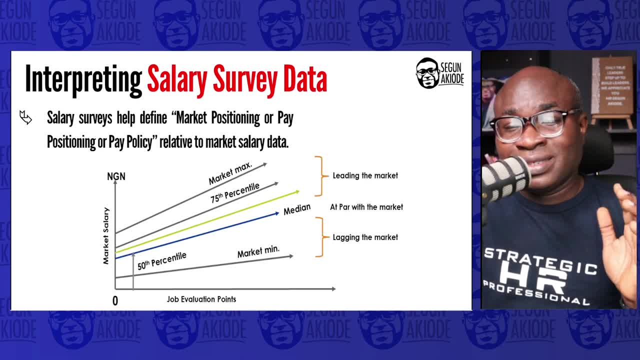 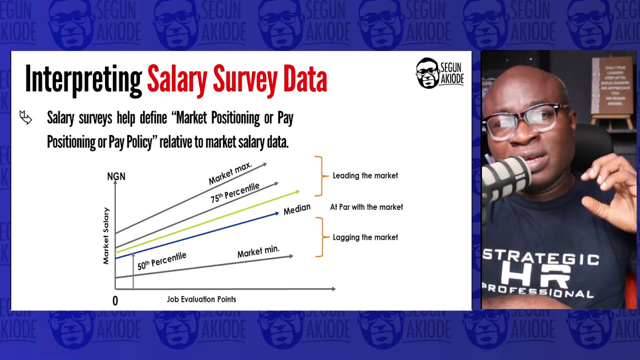 One is leading the market. two, being at par with the market and lagging the market. Now, for the sake of analysis, salary survey data are usually broken into percentile. Percentile is a statistical concept. that means dividing into 100 equal parts. Now, 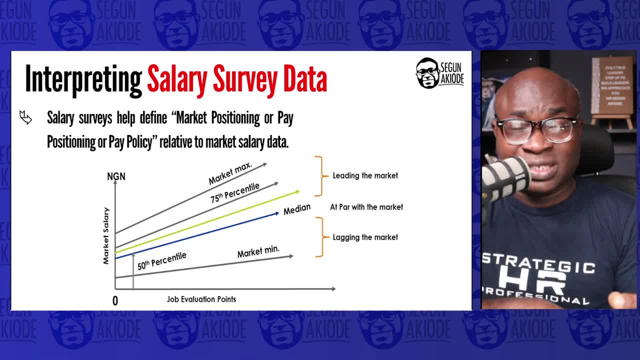 for 100 equal parts, it means the zeroth percentile is the lowest on the market, 50th percentile is the lowest on the market and the zeroth percentile is the lowest on the market. 100 percentile is the median of the market, while 100 percentile is the largest or the highest in. 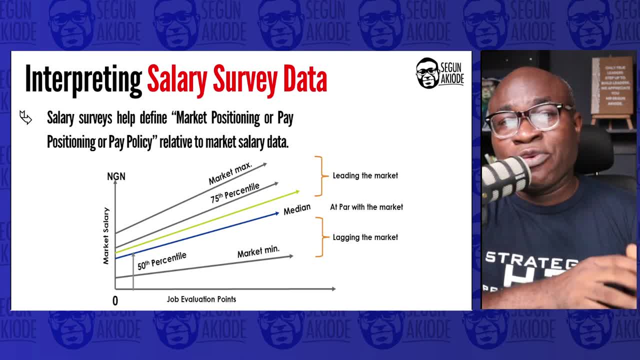 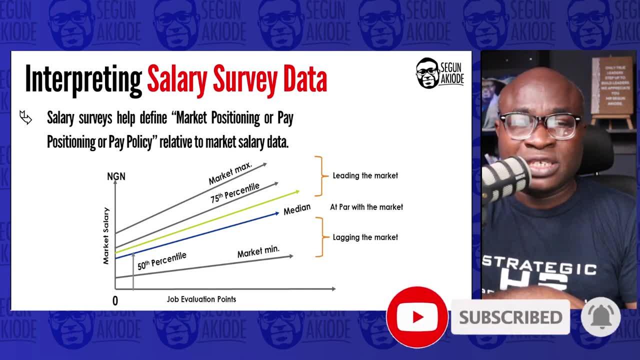 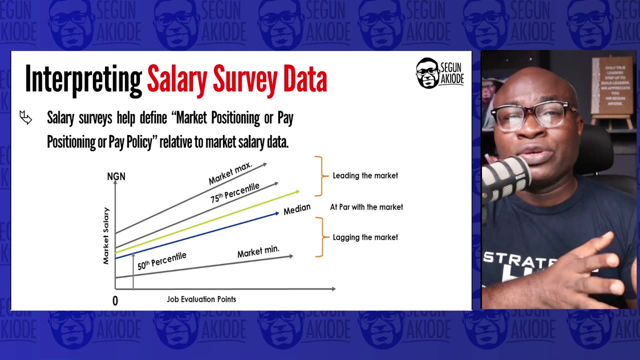 the market. Now, percentile in this scenario means leading the market is an organization pitching their salary above the 50th percentile of the market. Typically, let's speak, a Frontex executive that is currently earning 50,000.. Now, 50,000 is the market 50th percentile which is defined. 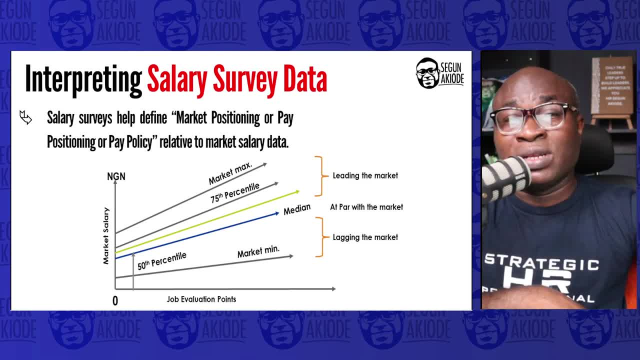 If an organization pitches a salary at that point it is at par with the market. If an organization chooses to pay more than 50,000, let's say 75,000, that organization is leading the market for that particular pay level for. 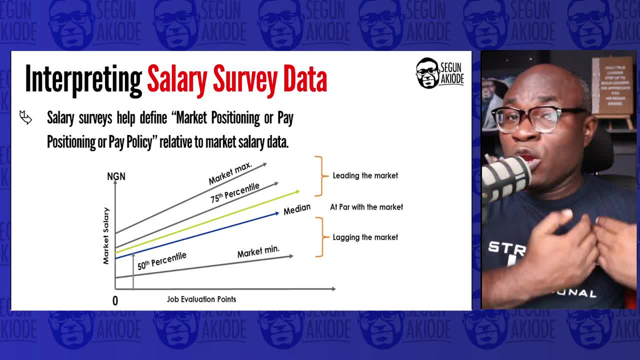 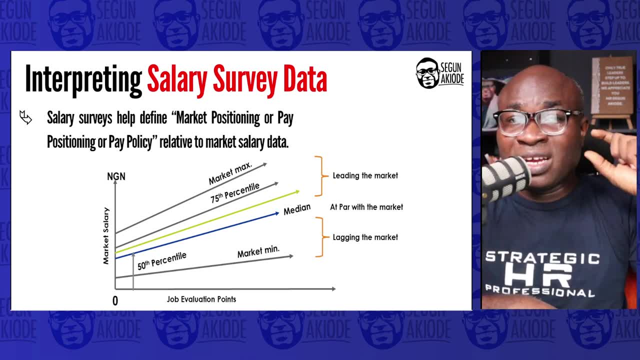 that salary And another organization that chooses to pay below 50,000, say 35,000, is actually lagging the market. So those are the three market positioning: leading the market, at par with the market and lagging the market. Usually when an organization 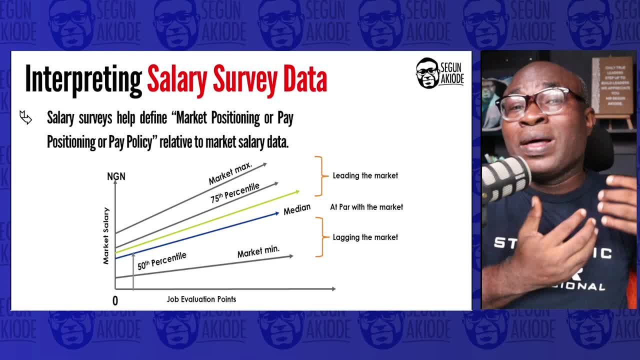 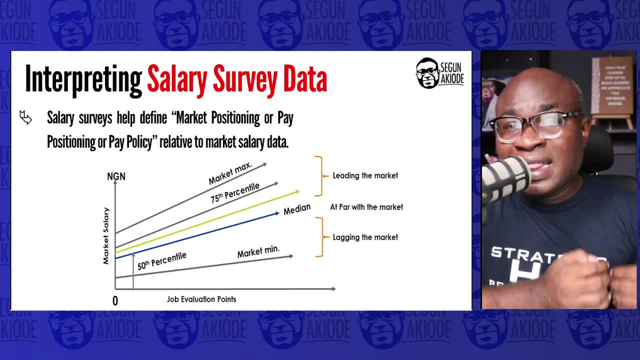 compares their own salary to the market 50th percentile, they will be able to know where they currently play in the market. Then they can be able to adjust their salary to determine any of these three positioning to take. We're going to get into Excel and I'll do a quick. 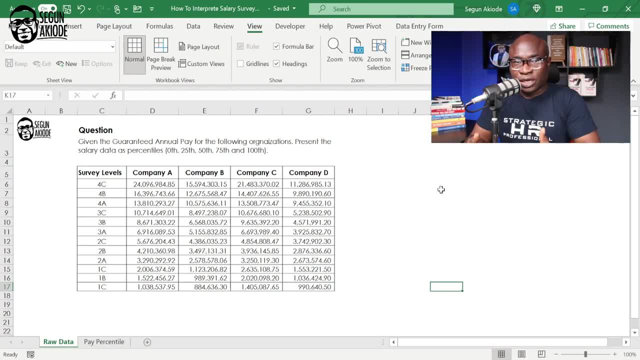 illustration. So let me quickly do a quick illustration. This particular example that I'm using to illustrate how to interpret salary survey data is actually a case study that we usually use in the compensation and benefit masterclass that I usually facilitate for Crescita Academy, And I'll be using that illustration for today. 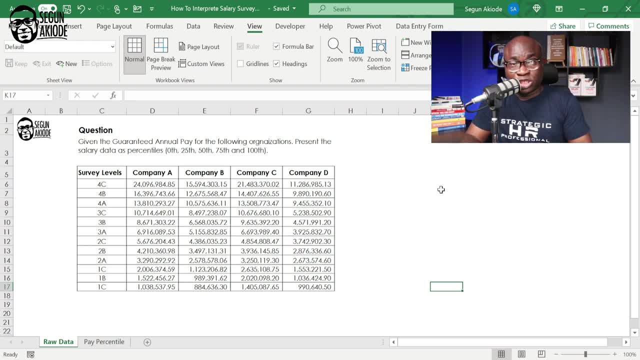 just to drive home the point around the pay positioning in terms of leading the market at par and lagging the market. So this particular question: you're giving the guaranteed annual pay for the following organization. The salary data is presented, So you have company A, B, C and D. The data has been collected. This 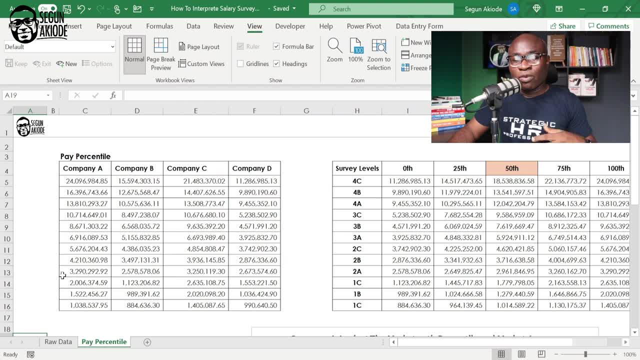 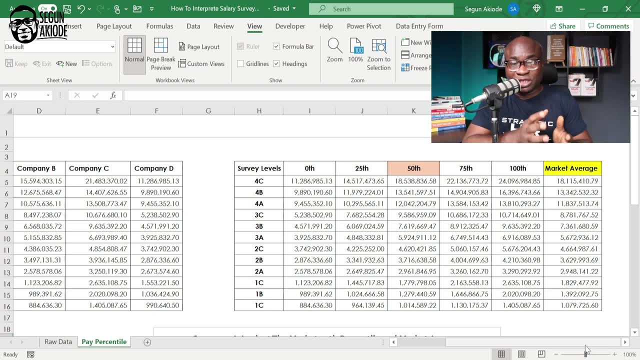 particular data is for fixed pay. Now, the pay percentile, in terms of what your normal salary analysis will have been done, is that each of the salary data from each of the organization would have been created as a percentile, And that is from your zeroth percentile to your hundredth percentile. 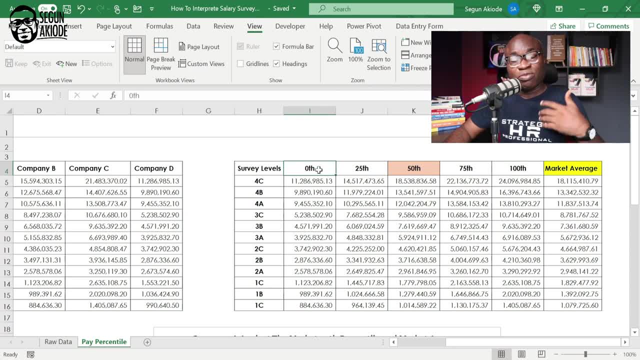 And for a lot of people it's going to be a lot of money. So you're going to have to do a lot of illustration purposes. You have your zeroth being the lowest in the market: 25th, 50th percentile. 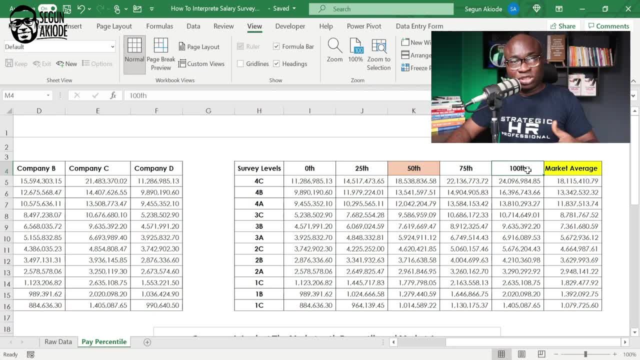 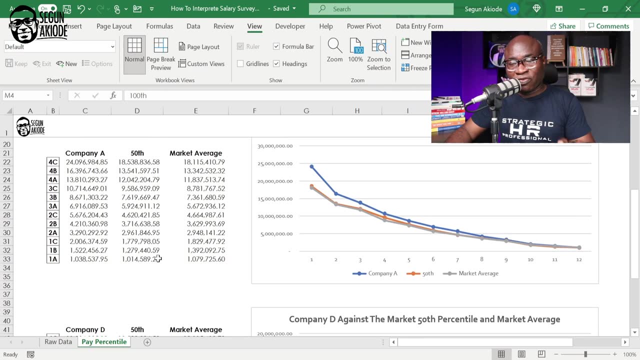 which is the market median 75th and the hundredth percentile. Now that is the data that has been presented in terms of the survey data itself. Now, if you now want to start to create positioning of each of the organizations, So for illustration purposes I've done a plot of company A in 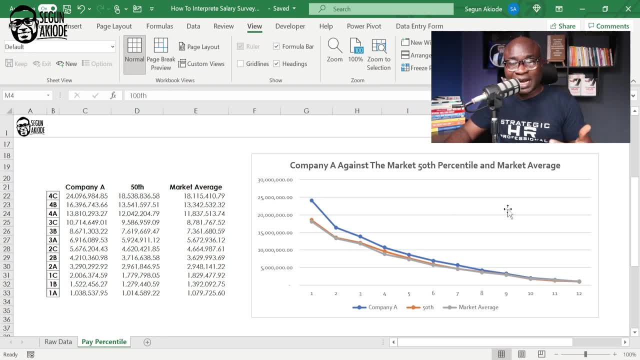 comparison to the 50th percentile. Now you would see from this particular plot of company A against the market 50th percentile and the market average, and you will see, ideally, that company A is the blue And you would already see that at each of the survey points, company A is actually leading in each of this point. That's why you see it's above the 50th percentile, which is the orange bit of it. 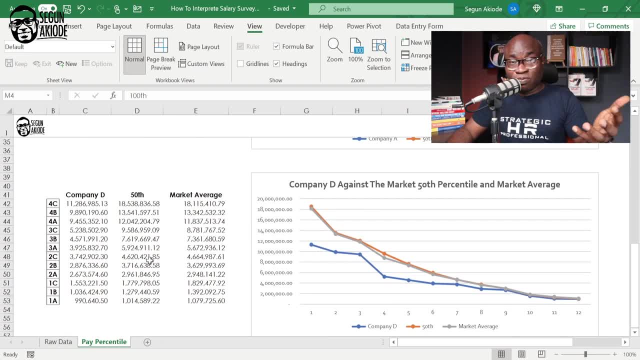 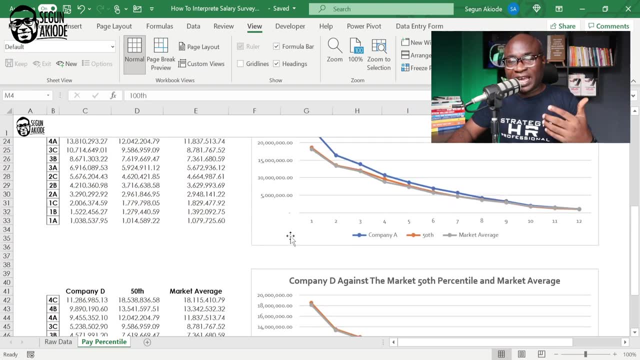 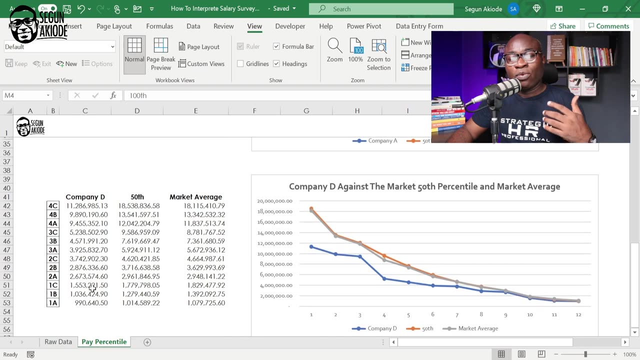 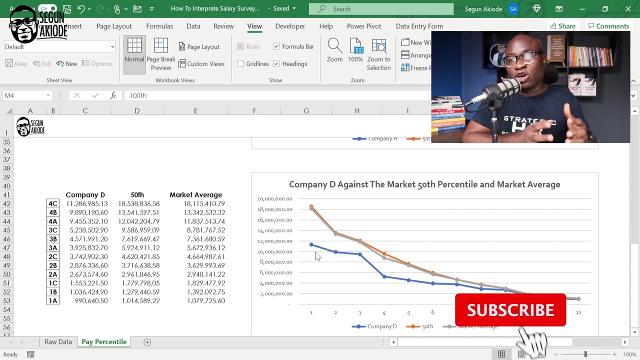 Then if I pick another organization- company D in this survey- result in themselves. you would see from the illustration that in the case of company A, they are leading the market in terms of the 50th percentile. in this scenario, Now, in case of company D, they are actually lagging the market because when you check them in comparison to the market 50th percentile, they are lagging the market. 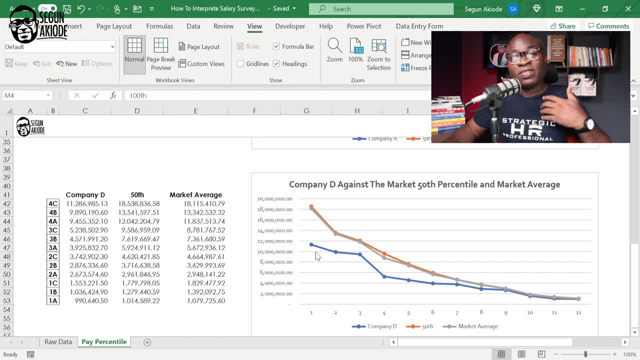 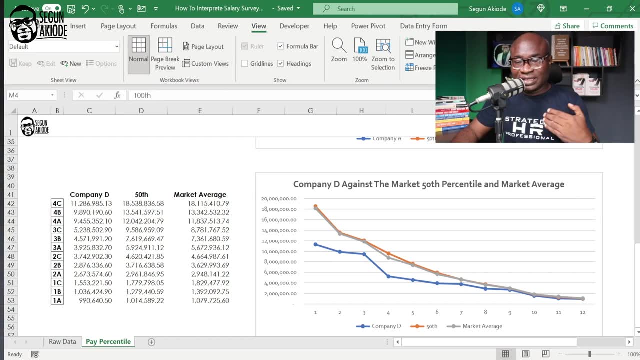 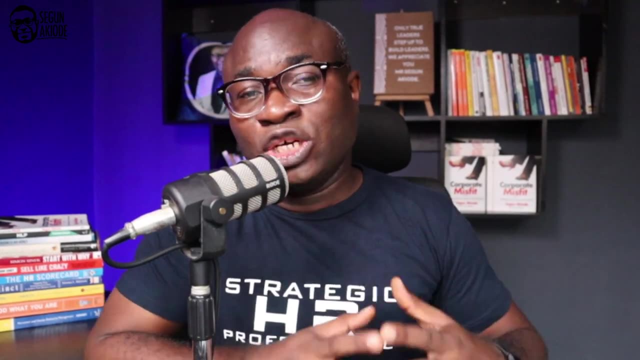 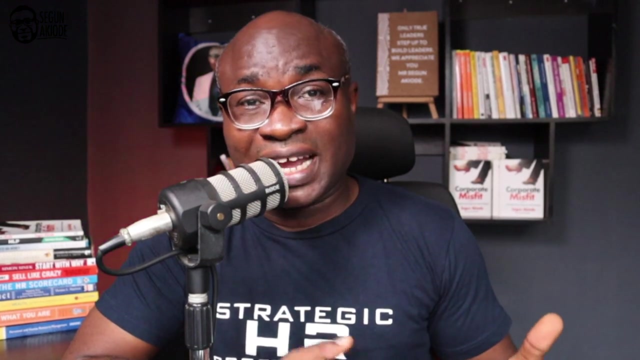 Now this is a typical example of a salary survey data trying to interpret how you would actually take a decision Based on the outcome of the salary data analysis which I just showed in Excel. now the organization will now be able to take a market positioning. If they find out that, if they compare themselves to the 50th percentile of the market, they are currently leading the market, they can decide to say: we want to continue to lead the market. 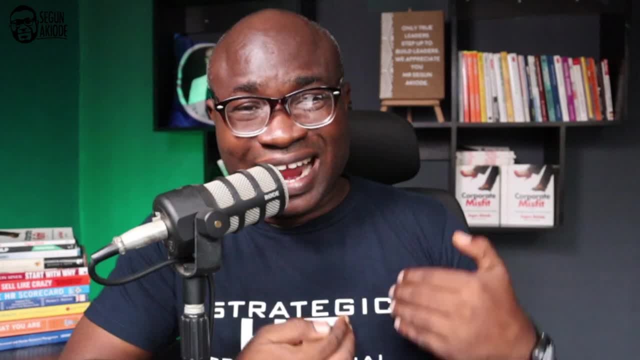 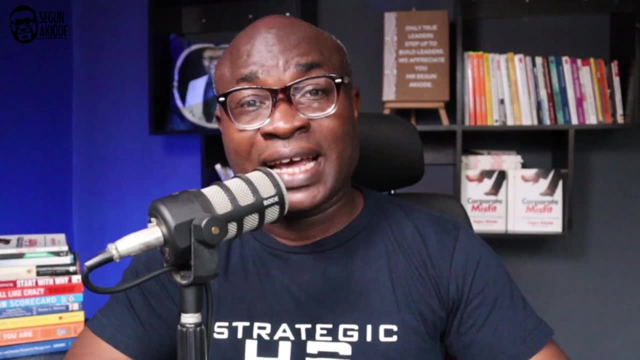 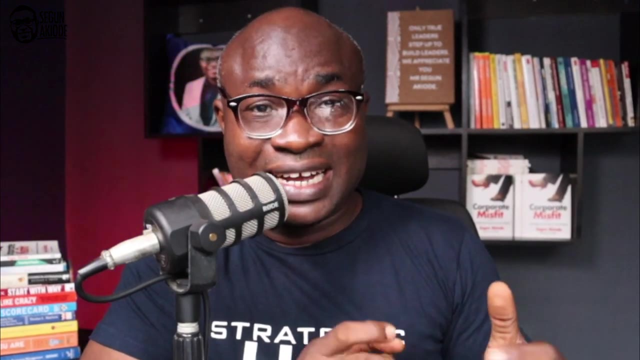 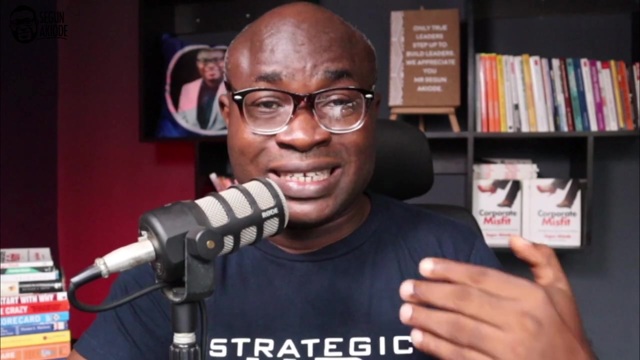 If they do that comparison, like company D in that example, and they are lagging the market, they can make a decision that want to move ourselves to the market average, which means they want to be a part of the market or they want to lead the market. Now each of the pay policy decisions that are decided would have an influence on the wage bill in itself, because the market movement will result to a salary action across the entire pay structure. 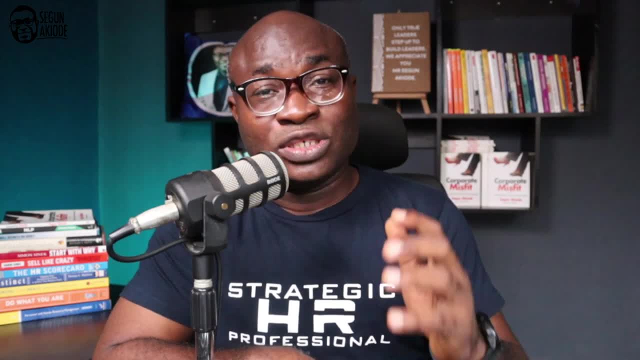 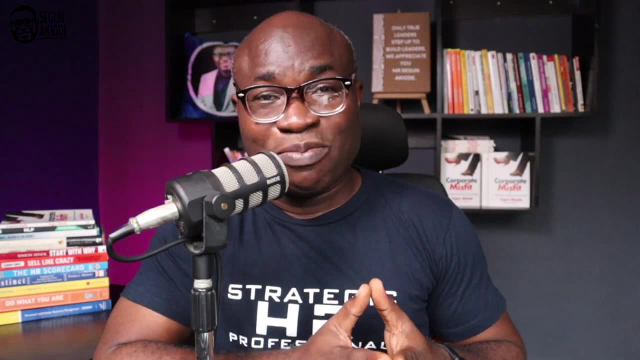 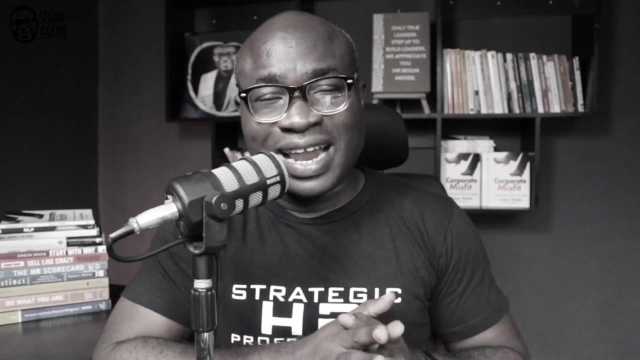 So there you have it, giving you a snapshot Of how to interpret salary survey data By adventure. you have any question for me? I kindly use the comment section below to ask your question. I'll see you in the next episode. Remember to slash. 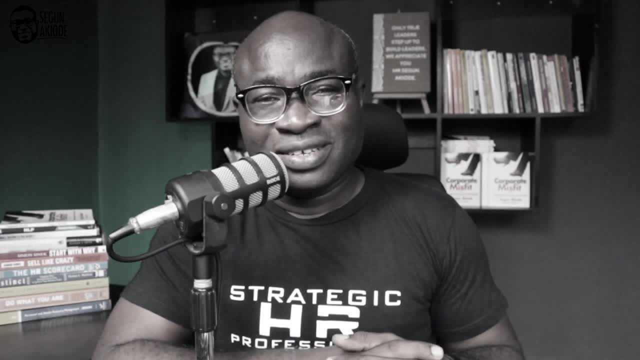 I'll see you in the next. Thank you very much. I'll see you in the next episode.